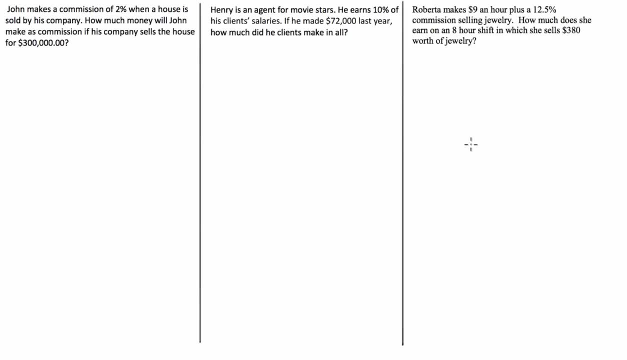 you're basically covered for most commission questions. They'll only be, like certain, I guess, changes or nuances different from these. So let's have a look at what we've got here. So we've got: John makes a commission of 2% when a house is sold by his company. 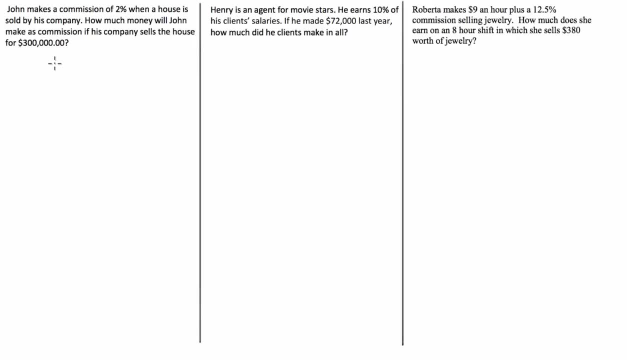 How much money would John make as commission if the company sells the house for 300 grand? Okay, so basically, the way that you work this one out is you go the value of the sale, which in this case is the value of the sale. So you go the value of the sale. 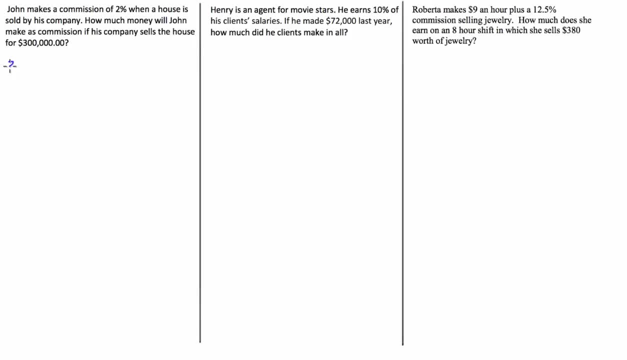 which in this case is 300,000.. And we multiply that by the percentage commission. Now, what I'm going to do in this case, guys, is I'm going to write it as a fraction, and I'll show you why in a second. 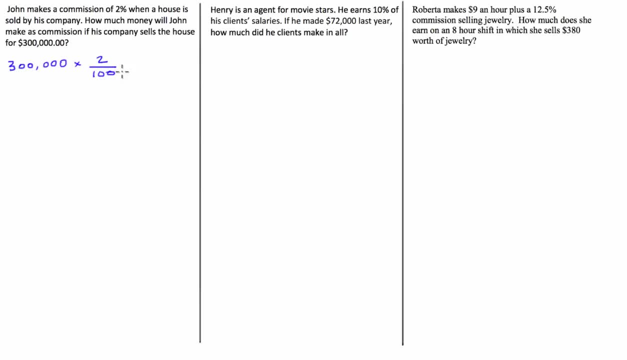 So we have 300,000 times 2%, which can be written as 300,000 times 2 over 100.. Now this, guys, we can write 300,000 times 2,, which is 600,000, divided by 100,. 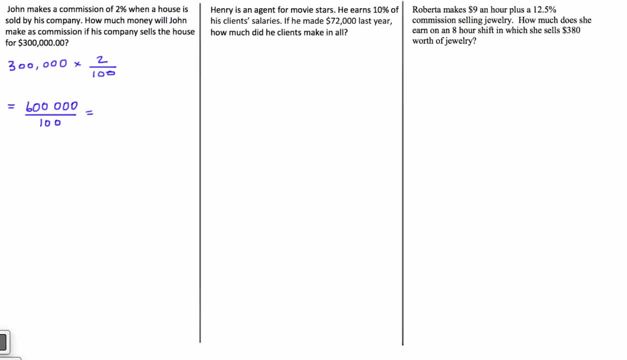 which is equal to. So the zeros we have two zeros cancel out, And what we have remaining is 6,000 over 1, or simply $6,000.. Now, what I would do, guys, is, if you're going to do these sort of commission questions, 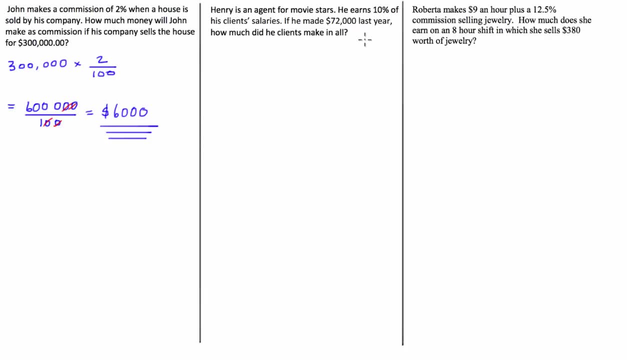 it's a good practice exercise to try and express the commissions, or the percentage commissions, as fractions. So then you can work a lot of these out without using a calculator. So let's go on to the next one. Henry is an agent for movie stars. 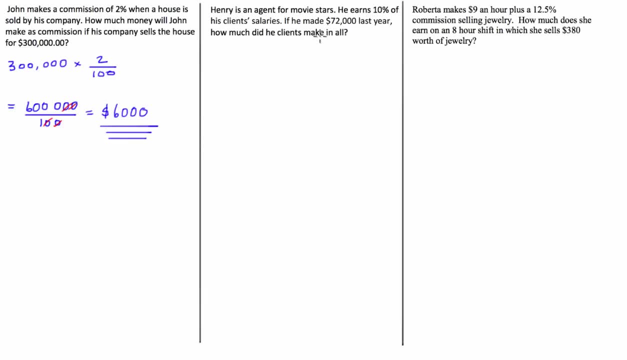 He earns 10% of his clients' salaries. If he made $72,000 last year, how much did his clients make in all? Okay, so what we're going to do is we're going to call the amount that his clients made. 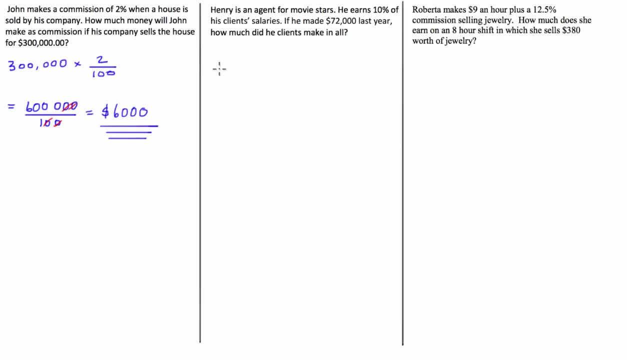 we'll call that C. So C dollars times 10%, like we have over here, is equal to $72,000.. Cool, so hopefully you guys know a little bit about algebra. So we're timesing this 10 over 100 by the salary of all of his clients. 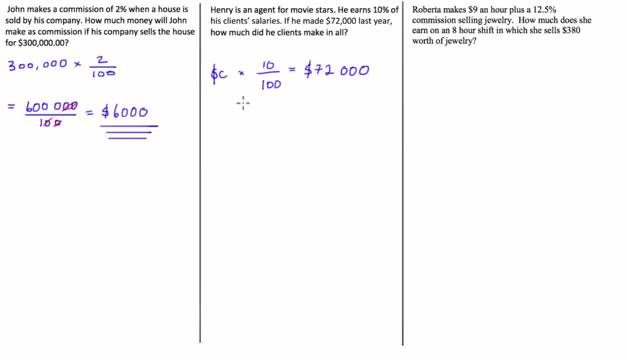 So to move the 10 over 100 to the other side, we're going to divide both sides by 10 over 100. And what ends up happening is these will cancel out And we'll be left with: C dollars is equal to $72,000. 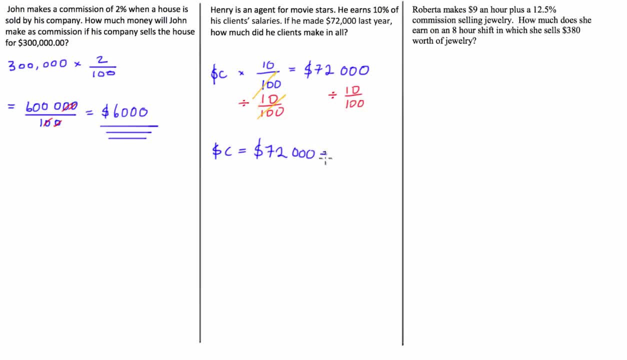 divided by 10 over 100.. Now, with fractions you can't divide a number by a fraction. It just doesn't work. So what we do is, when we're faced with a division by a fraction, the division by a fraction is simply multiplication by the reciprocal of that fraction. 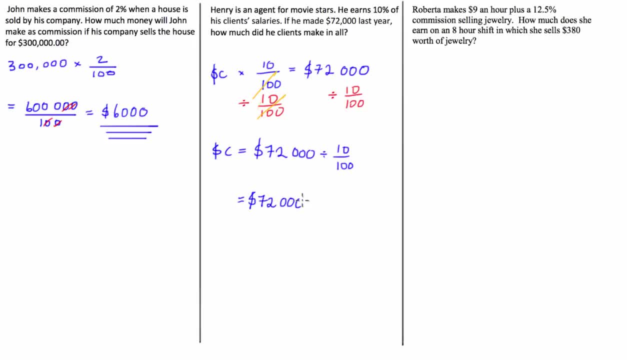 So we're going to have $72,000 times 100 over 10.. Now 100 over 10 is just we can just times that by 10.. So 72 grand times by 10.. Hopefully you guys understand that that's going to be. $720,000.. Cool, Now Roberto makes $9 an hour, plus 12.5% commission, selling jewelry. So in this case here, both of these ones were both straight commissions, So there was no base wage or salary. They only got paid when they actually sold something. 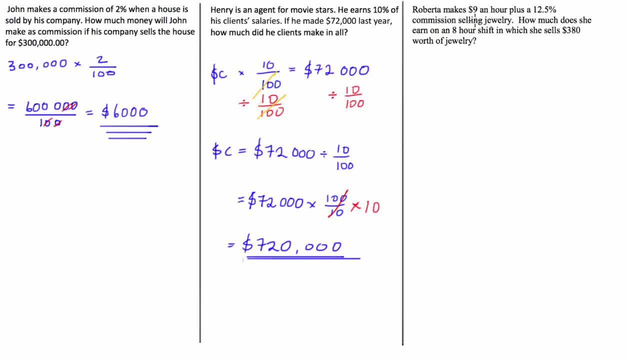 But this one, Roberta. she gets paid $9 an hour, regardless if she sells anything or not, So plus 12.5% commission selling jewelry. How much does she earn on an eight hour shift in which she sells $380 worth of jewelry? 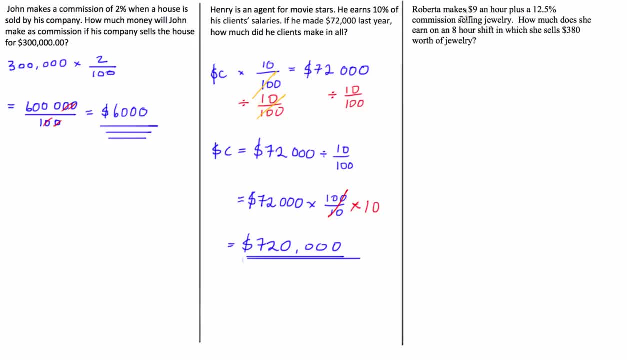 Okay, So well, let's write down what we've got here, because this is a little bit more complicated. this one, So. her take-home pay is equal to $9 per hour plus 12.5% commission. Okay, So what we have to do is I'm going to break this question down into her hourly rate, or? 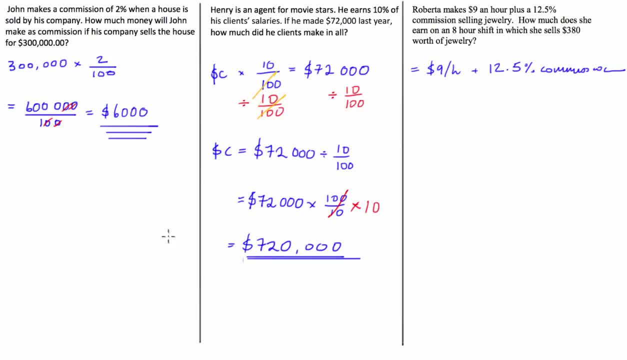 a total salary plus her total commission. I'll do both of them separately, so we can then add them together at the end. So let's start with her salary. Cool, So her salary is going to be equal to $9 per hour. times what. 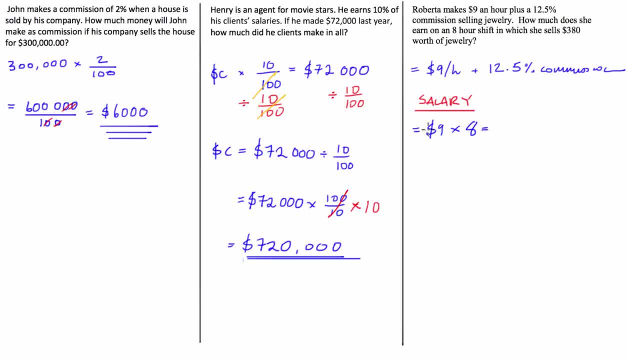 How long does she spend there? Eight hours, And that's equal $72.. Cool, Now we're going to work on her commission. So, like we did in this one here, the commission is going to be the total amount she sells multiplied by her percentage commission. 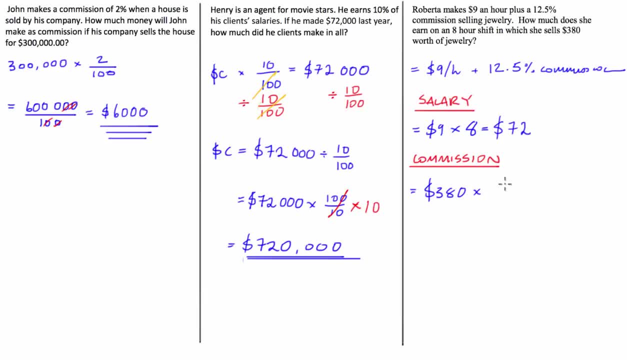 Now I'm going to write that as a fraction, like I've done in each one of these. So it's going to be 12.5 divided by 100.. Now, 12.5 divided by 100.. This can be simplified to 1 over 8.. 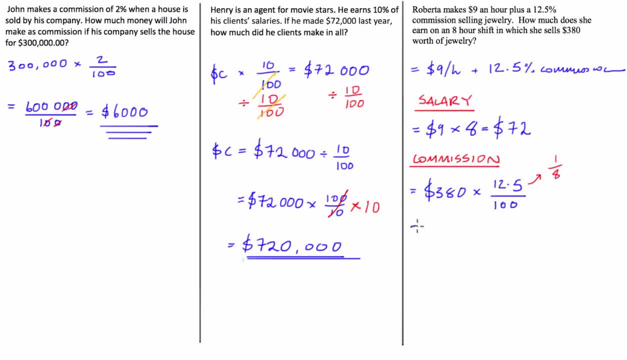 So that's what we're going to write it as. So we have $380 times 1 on 8.. So this is equal to $380 on 8.. Now I've got space over here, So I'm going to work this number out. 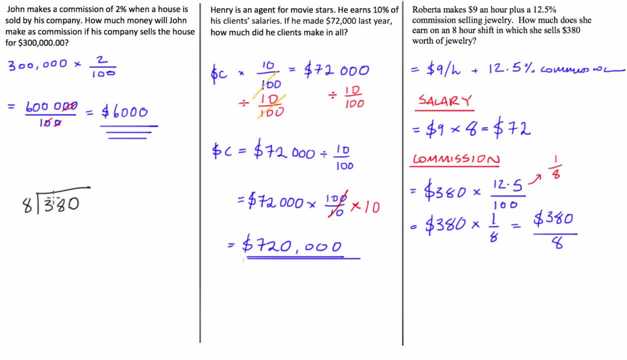 Cool. So 8 to the 3 can't do. 8 to the 38 goes 4 times, That's 4 to the 32.. Remainder: 6.. 8 to the 60 goes 6.. 8 to the 56.. 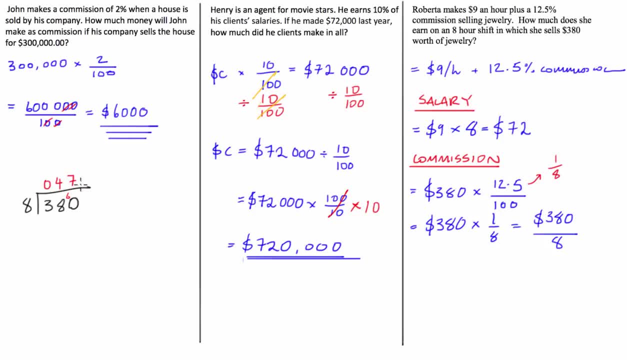 6 to the 48.. 7 to the 56. Remainder 4.. 8 to the 40 goes 5 times. So this is going to be equal to- Let me just bring that back- $47.50. So our total pay: 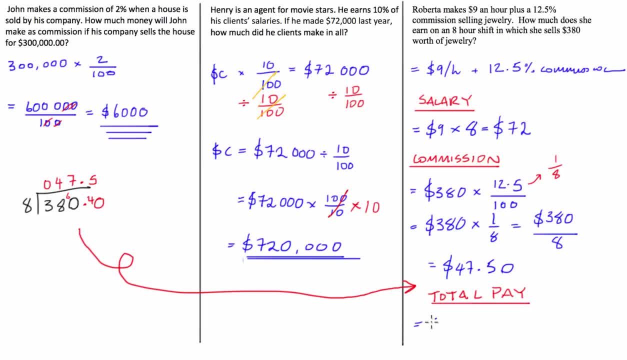 This is going to be equal to $72.00.. Plus $47.50.. Which is equal to $119.50.. Okay, so obviously this one here was the most complicated. However, they all basically require the same strategy when you start. 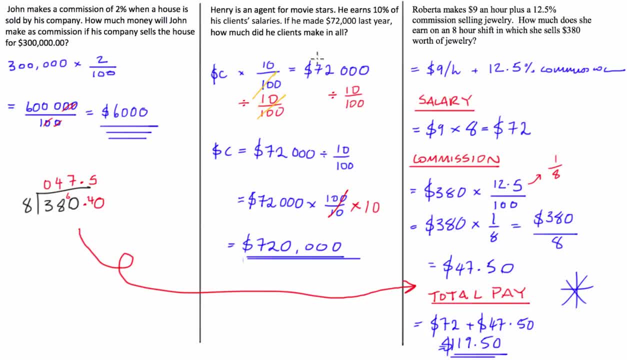 You set up the equation, The percentage commission that the employee will receive. So what we have here, We have the employee, So this is what the employee will receive, And we have employer on this side, What the employer will receive from the sales. 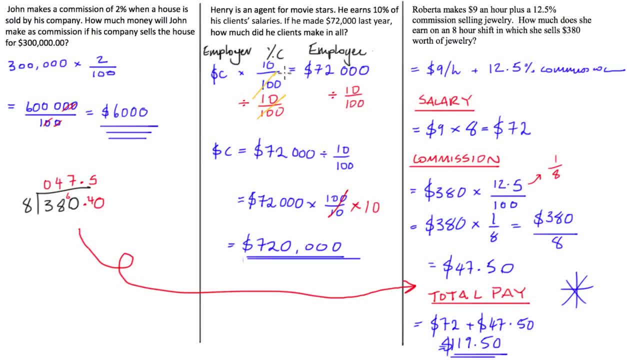 And this bit here is your percentage commission. So if you set up your equation like this, It doesn't matter if you have to work backwards or forwards, You don't have to rote, learn any special methods for working backwards. You can just set it up like this: 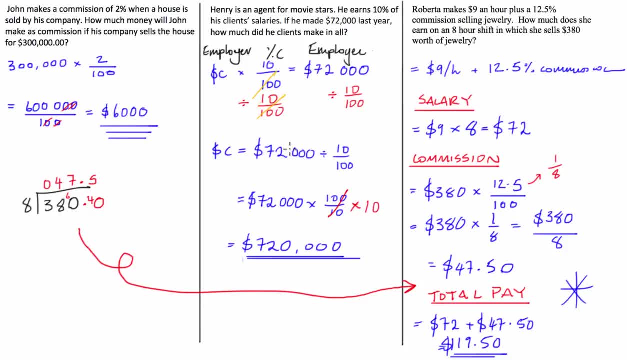 And then use algebra and a little bit of fractions to solve them. So I would practice it like that, Setting up the equations exactly the same each time And either going forwards or backwards Depending on what the question is asking. Remember when you do these: